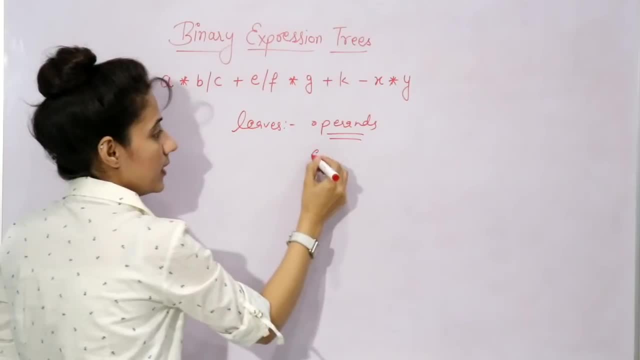 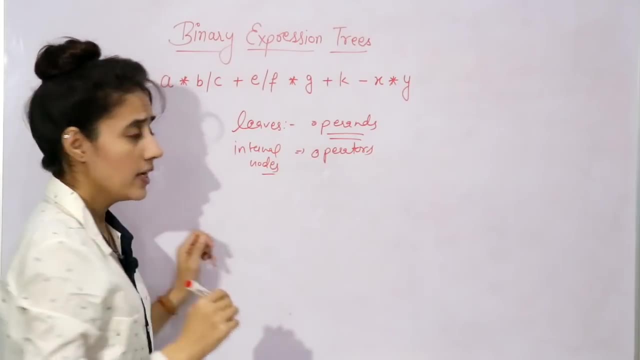 what you are going to store All the symbols. or you can say all the operators would be assigned in internal nodes. So you can say: expression tree is a tree in which each internal node corresponds to the operators and each internal node corresponds to the operators. So you can. 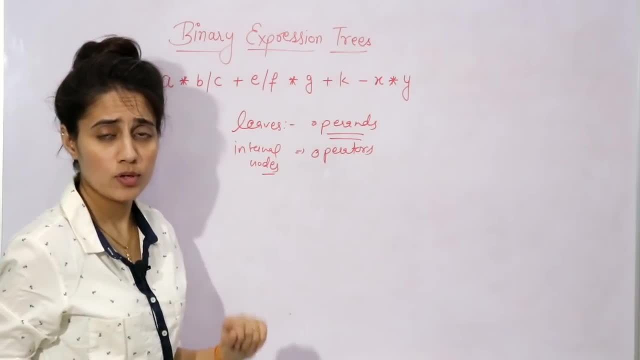 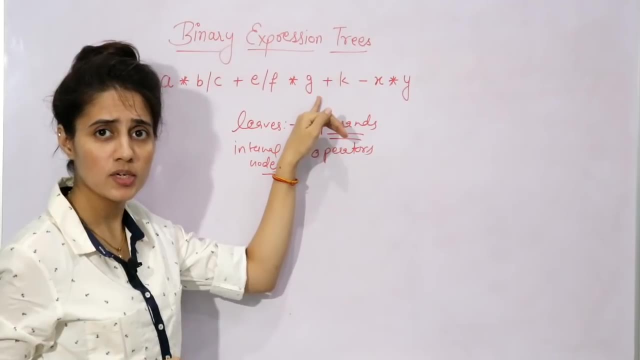 say, each leaf node would correspond to operands, or you can say would store operands. right Now we will see how to construct. If you are given with an infix expression, then can you represent this expression in the form of a tree. See, basically it is very simple to construct. 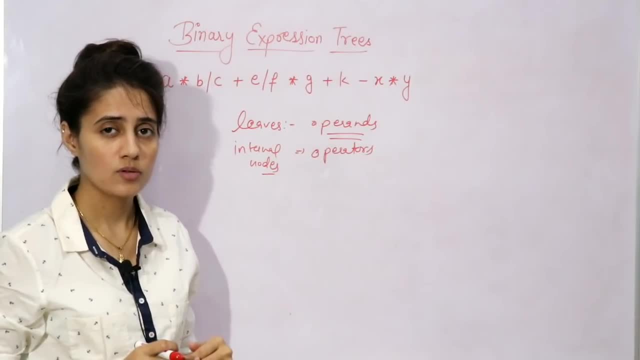 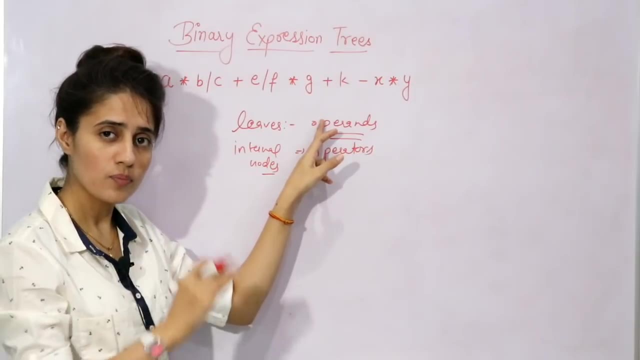 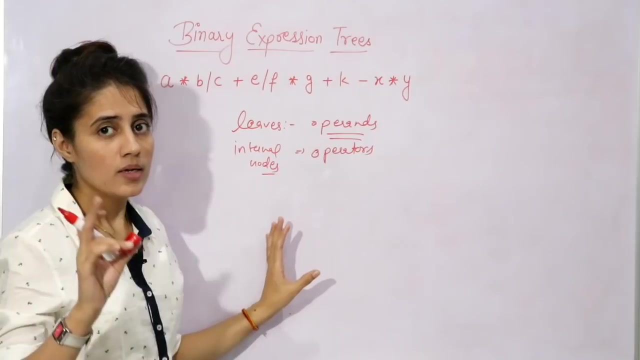 a expression tree with the help of postfix expression. So one method is you convert this infix expression into postfix expression. Then, using stack from that postfix expression, you can easily draw, you can easily construct an expression tree. But here in this video I am not going to. 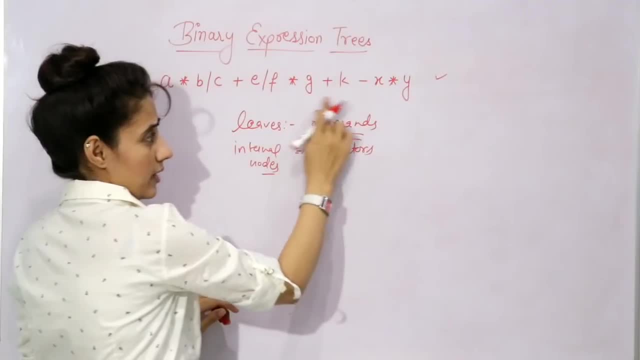 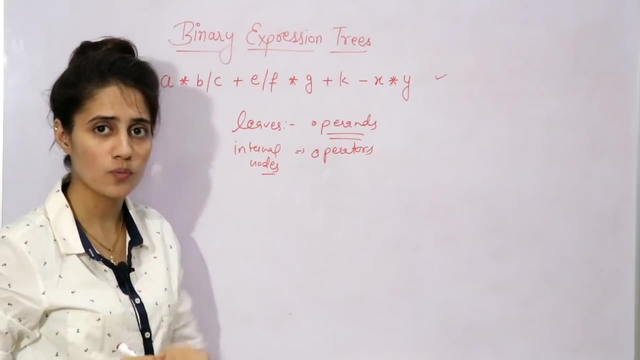 follow that approach. I will directly construct a binary expression tree from this infix expression only. We are not going to convert it into postfix expression. That thing we will discuss in the next video, right? So this would be a little bit tricky methods, fine, So you need to concentrate. 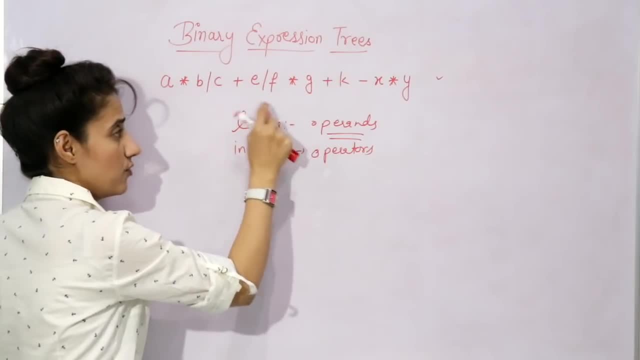 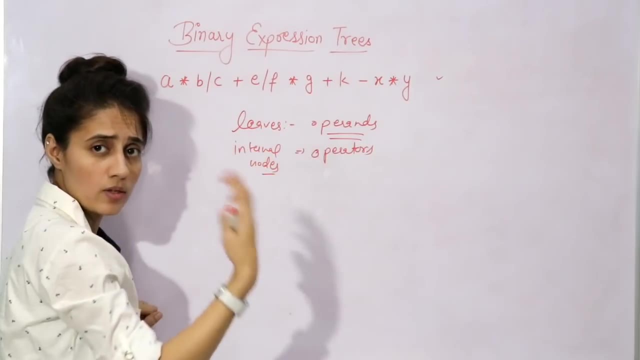 on this method. Now let us see how to construct the expression tree from this infix expression directly. We do not have any brackets, right? If there are brackets, then we are going to construct this. If there are no brackets in the expression, then also some another rules we are going to. 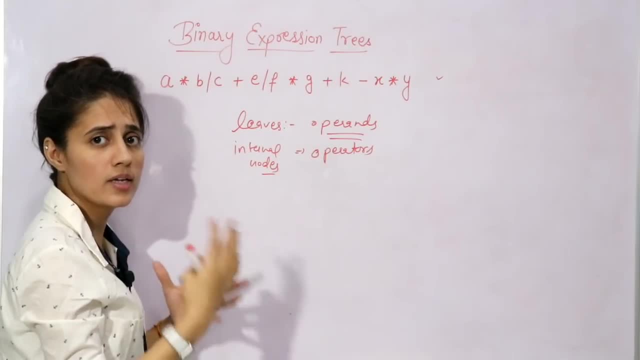 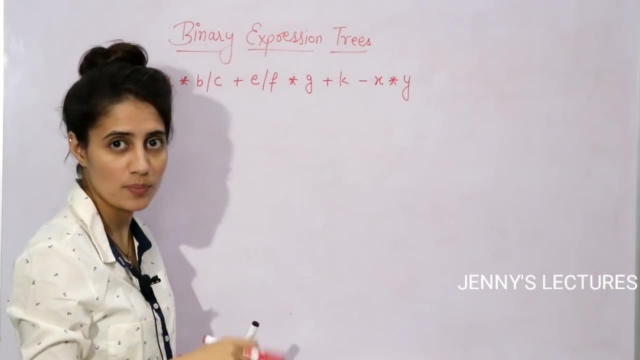 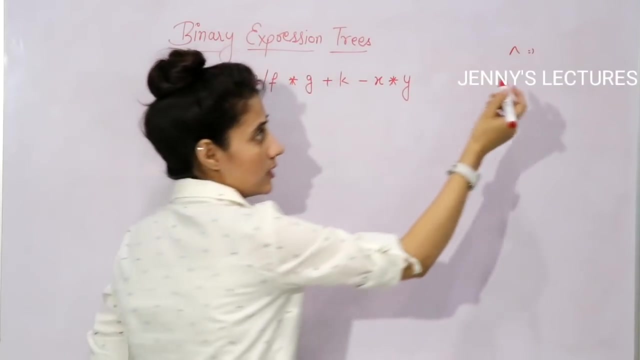 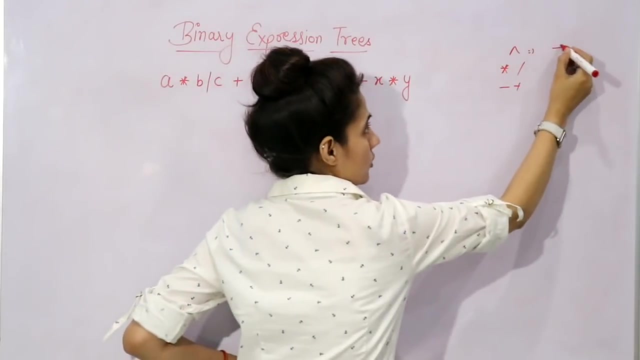 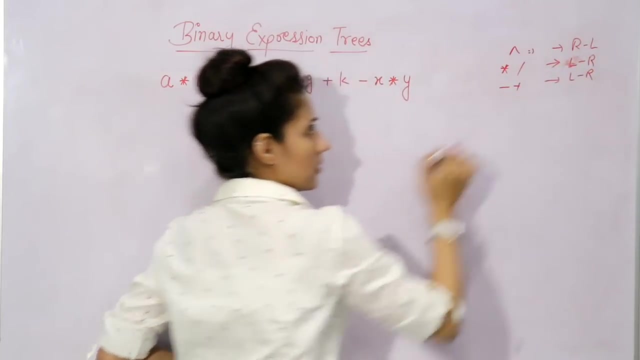 follow Rules would be same, but a slight difference would be there in case of, while we- Así que en este caso, como enTantas babe areosos is right to left. this is sorry, left to right, and this is also left to right. now how we are going. 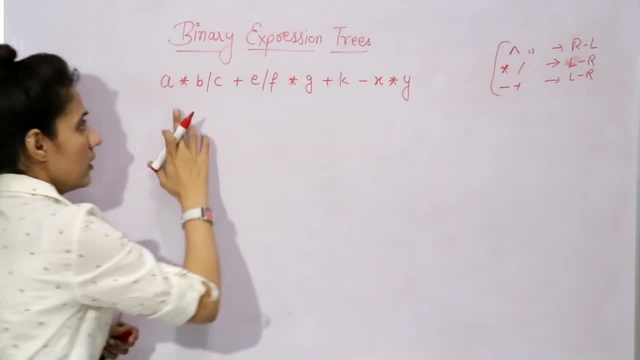 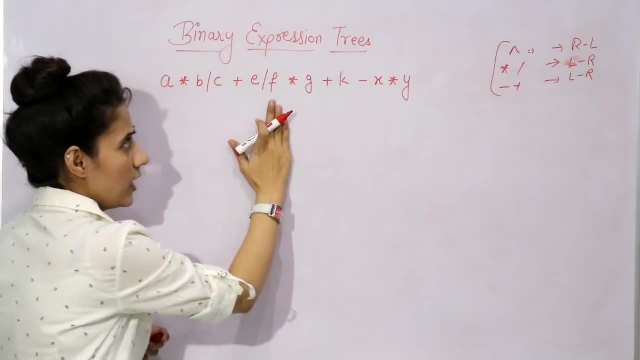 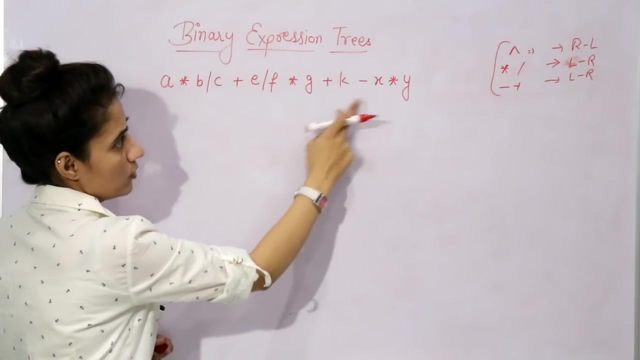 to use these rules that you need to take care now. see, the root would be what you need to take care of that thing. the root would be what? see, by looking at this expression, can you tell me which operator you will evaluate first? the highest precedence operator? here we don't have power. 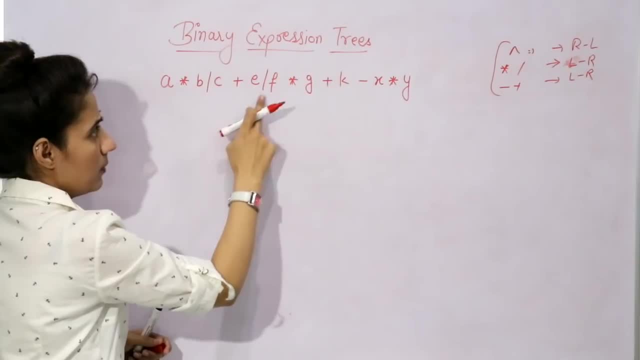 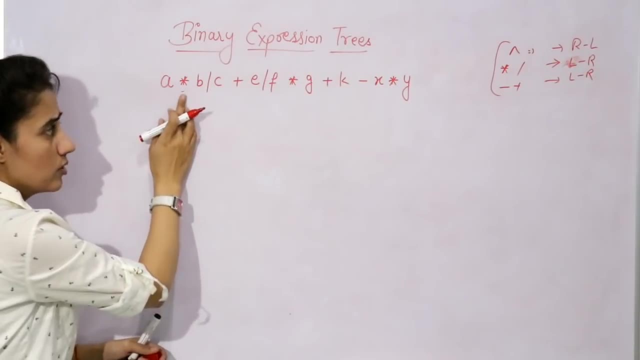 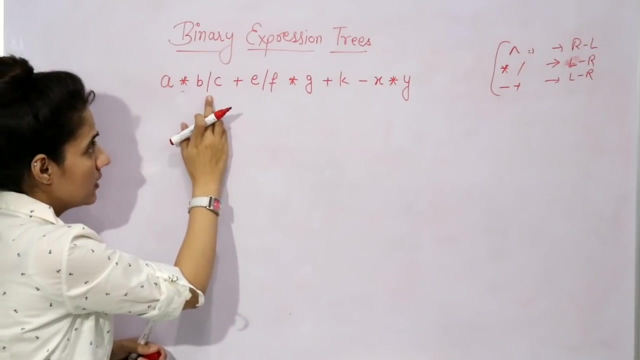 so we have here multiplication and divide, but here multiple multiplication and divide operator are there. so check out the associativity that is left to right, scan this from left to right. so this would be the first operator. that is first s trick. so we will evaluate this multiplication first, after this that this divide, then this divide in this and this, something like. 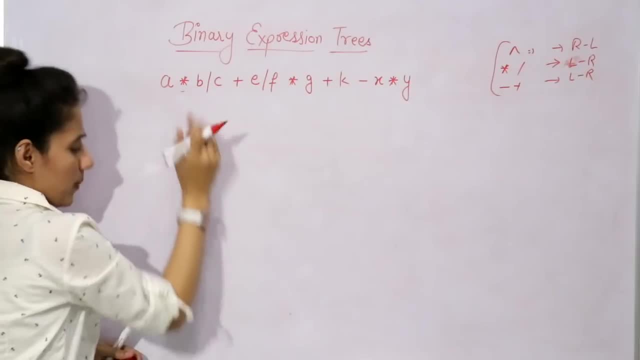 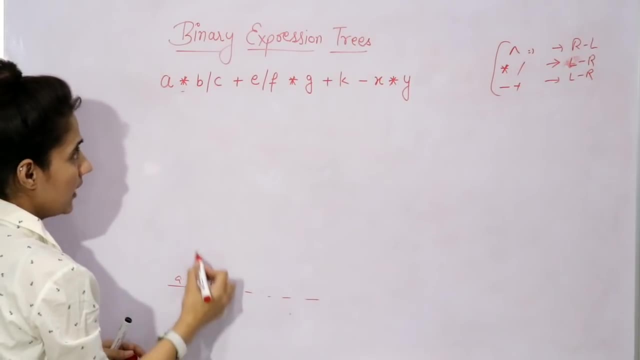 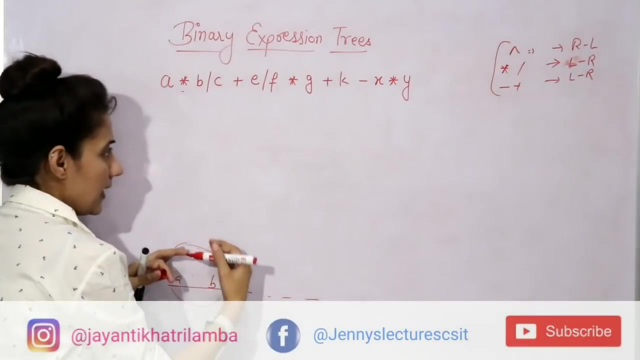 this right, but see, these operands would be here at the leaf node right. so now you can say: suppose here we have a and b, so here we have s tricks. so first of all, this should be evaluated right and at last, at last, means the operator which would be at the top, at the root of the 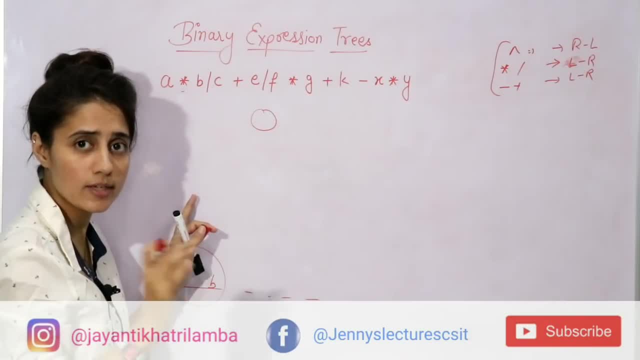 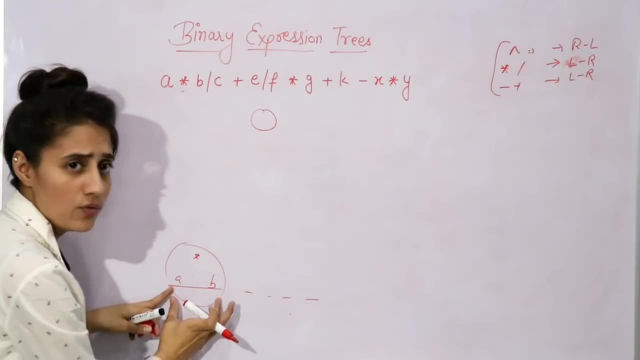 tree that would be evaluated at the last yes or no. by looking at this tree you can easily analyze this thing. first of all, we will evaluate from here, because here in the leaf node only we are having operands. so first of all we need to evaluate. we need to start the evaluation from the here. 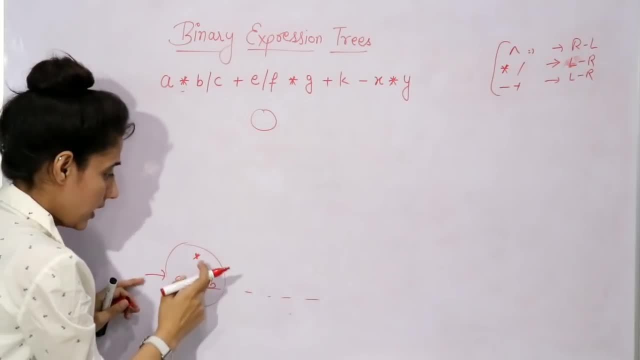 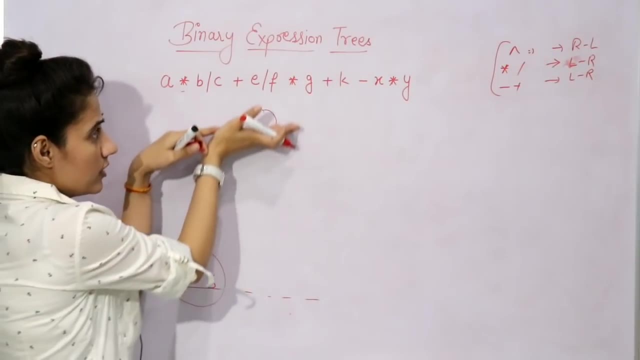 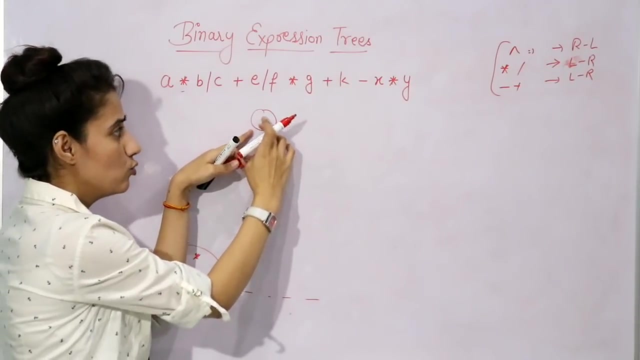 from the leaf nodes. so you can say higher precedence operator would be here, towards the leaf nodes, and the least precedence operator would be at the top, because this at the root, you can say at the root, the least precedence operator would be at the root node of the tree. 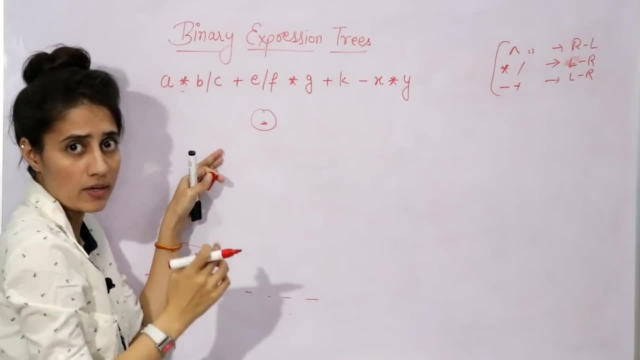 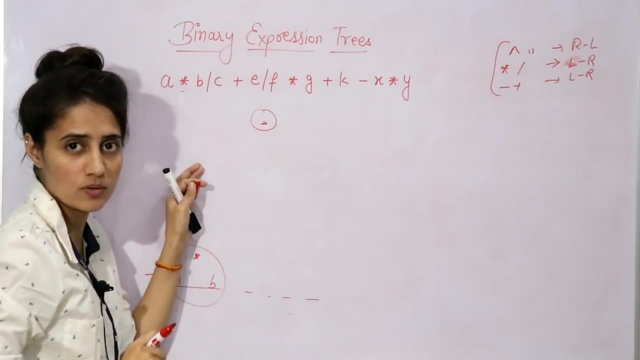 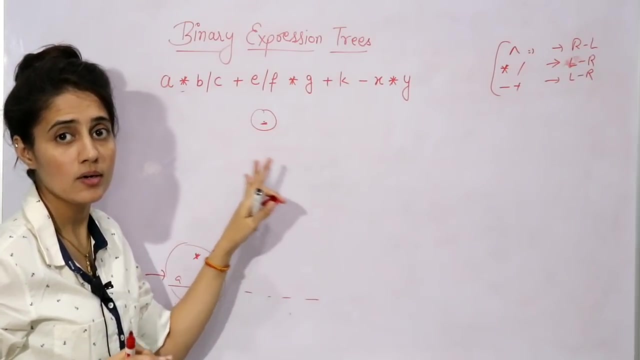 because this would be evaluated at the last right and obviously the rule is the least precedence operator we are going to evaluate at the last in the sinfix expression right. so So what you need to take care of: find out the least precedence operator from here while constructing a expression tree from the infix expression right. So now, the least precedence. 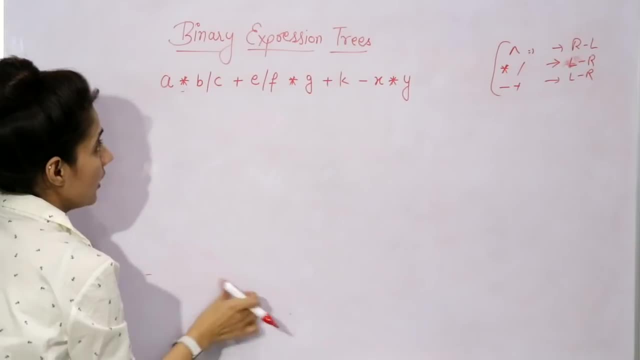 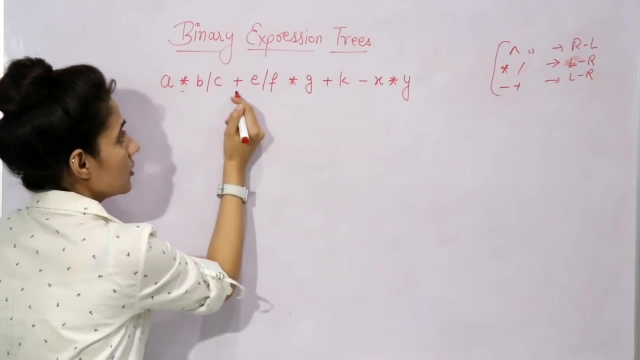 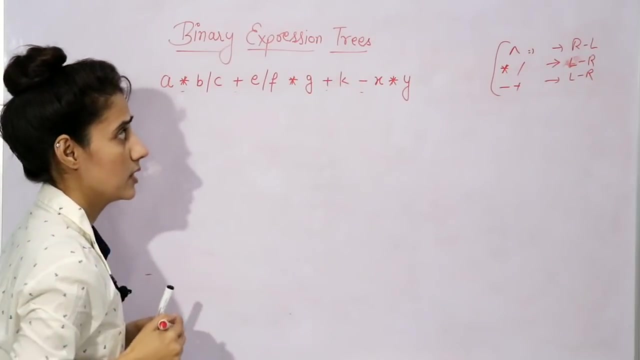 operator is plus and minus, but here we have plus and multiple times plus and minus. So now also, you need to find out which you are going to evaluate at the last, this plus, this plus or this minus. because we have 1, 2 and 3. these operators are having same precedence. Now check out the. 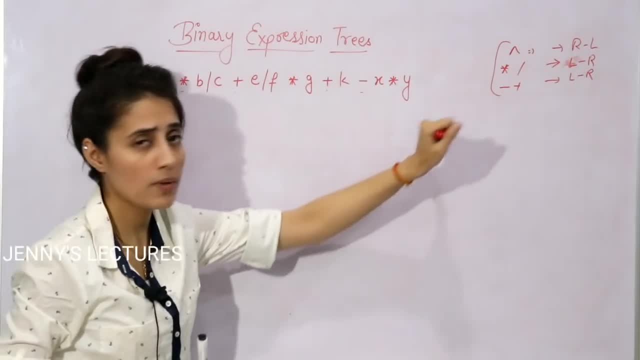 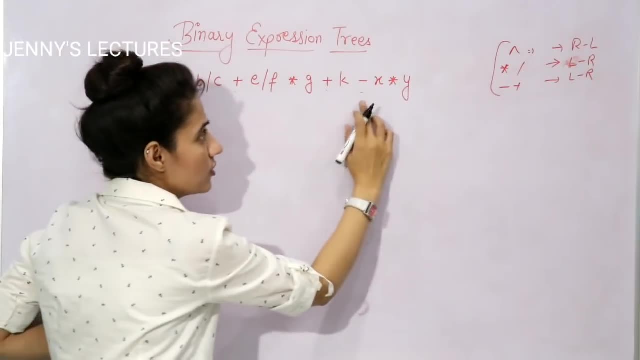 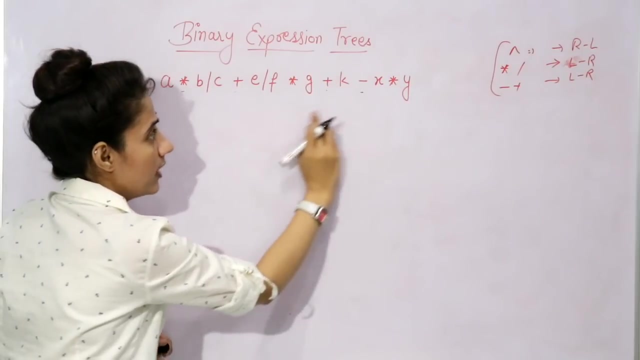 associativity. Associativity is left to right. for this plus and minus. Now scan this from left to right, right, and at last we have this minus, because while scanning from left to right, this would be the first, so we would evaluate this first, then we would evaluate this plus, then we would evaluate. 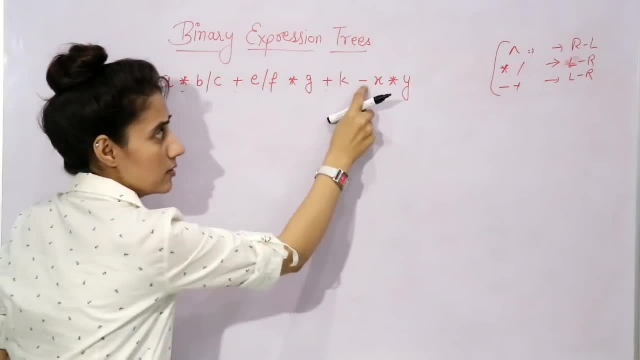 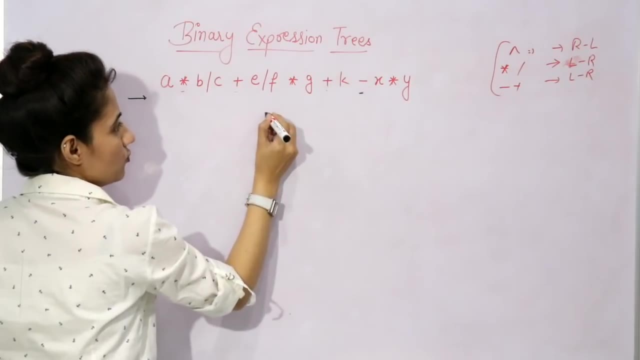 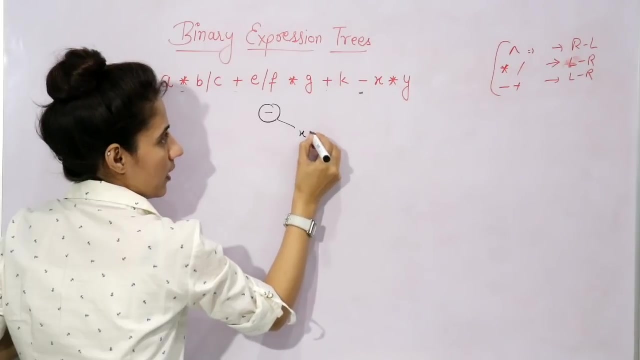 this minus means this would be evaluated in the last. this minus Right, it means we have found a root, root of the tree. So now this minus would be the root of the tree, right. So now this part would be the right part of this tree, or you can say the right subtree. 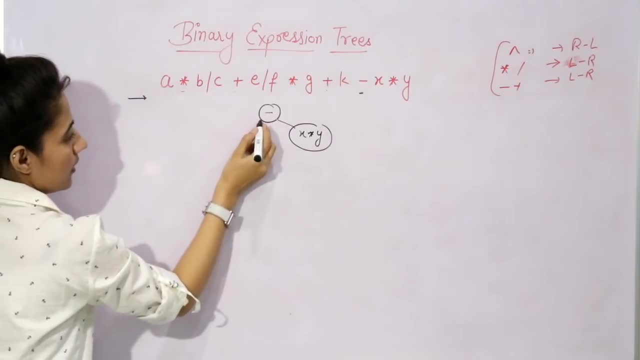 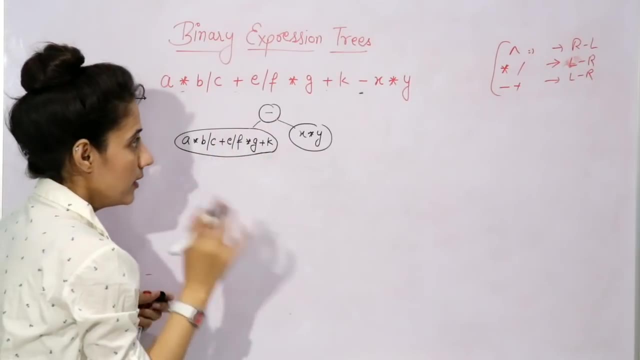 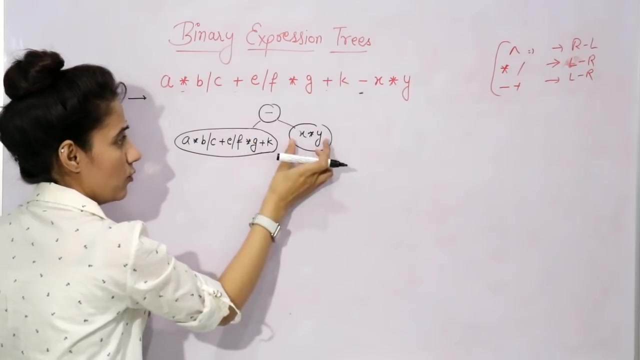 of this tree and this complete would be the left one. So this is the left and this is the right subtree. right Now we have broken this Infix expression. Now we have two sub infix expressions. One is this one, one is this one. 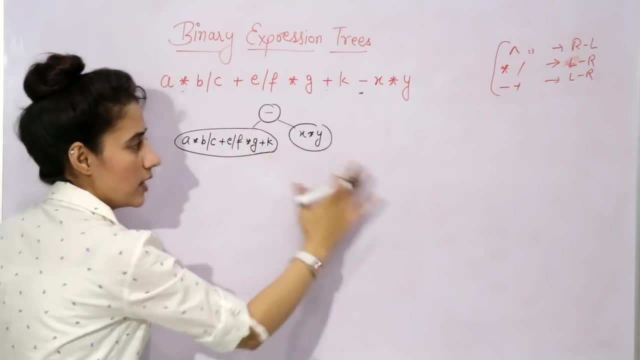 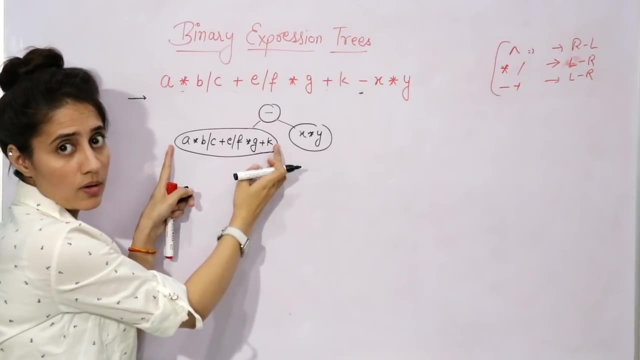 So you can now. we will construct first of all the left subtree, then the right subtree. You can construct right subtree also. it's up to you. Now again, apply the same rule here also: Find out the operator which is having minimum precedence. That would be the root, right from. 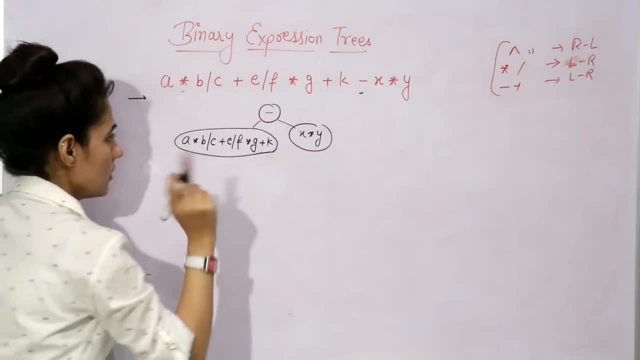 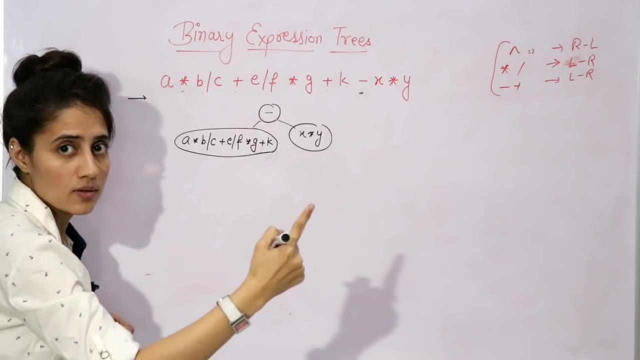 where we are going to split this expression right Now. here also, plus Plus is having least precedence, but which plus you are going to split this expression right Now? here also plus Plus is having least precedence, but which plus you are going to evaluate in the last. That would be the. 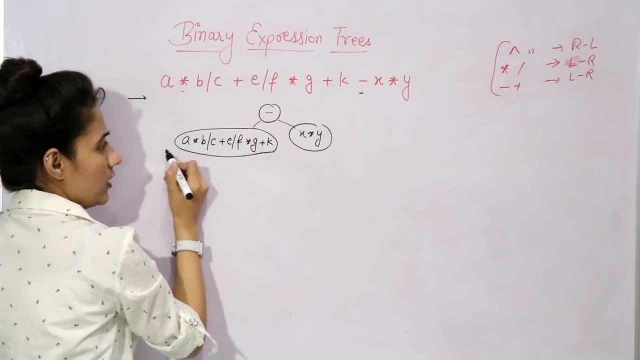 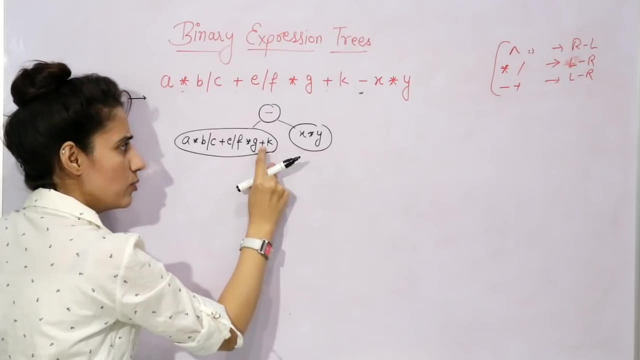 root for this subtree, na For the left subtree. So now scan it from left to right, because associativity is left to right. So while scanning, this would be evaluated, evaluated first, after that this one. So it means this plus would be evaluated at the last in this subtree, in the, this expression. 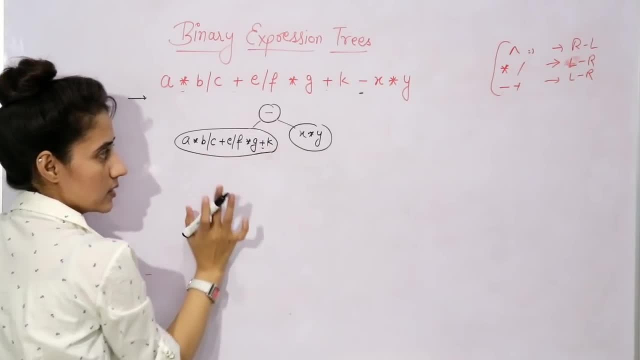 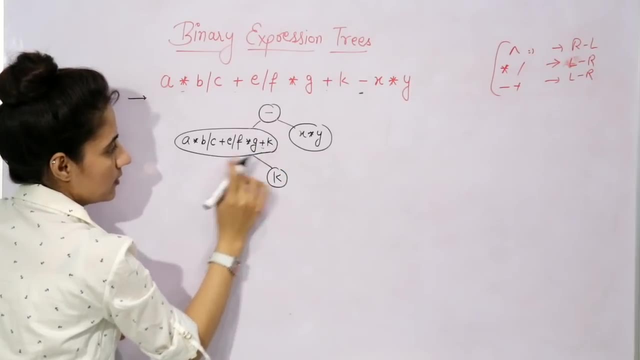 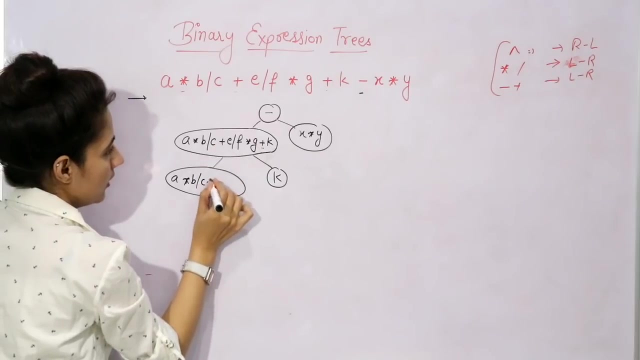 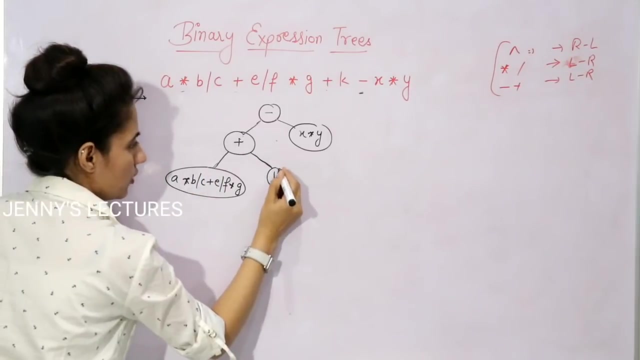 So this would be the root. from here we are going to split this. Fine, So this k would be the right subtree and this is what You can say. left, This complete expression would be left subtree, part of left subtree, And here the root is what plus only Now, this is the subtree. Now again, check left, end right. 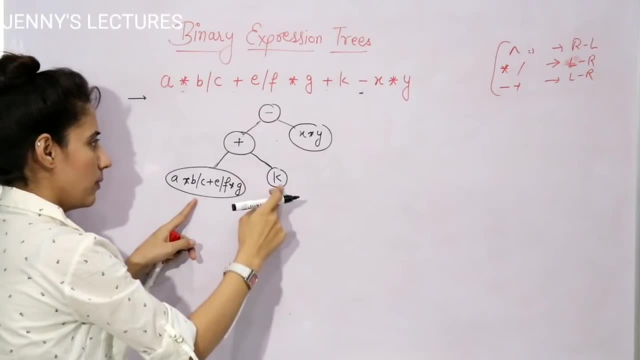 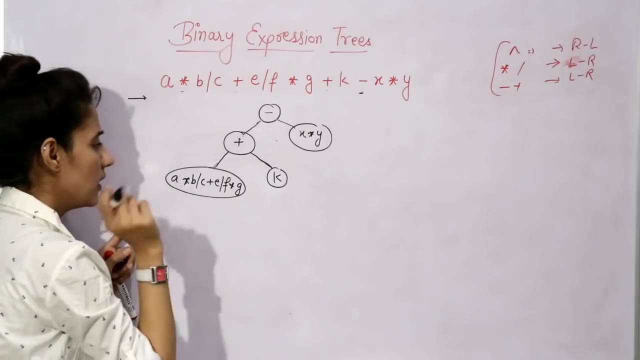 subtree. Here we have operand, So this is the leaf node, So no need to bother about this thing. Now we will construct this left subtree for this expression. Same rule we are going to follow: find out the operator which is having least precedence, That is, plus. We have only one plus, So we are 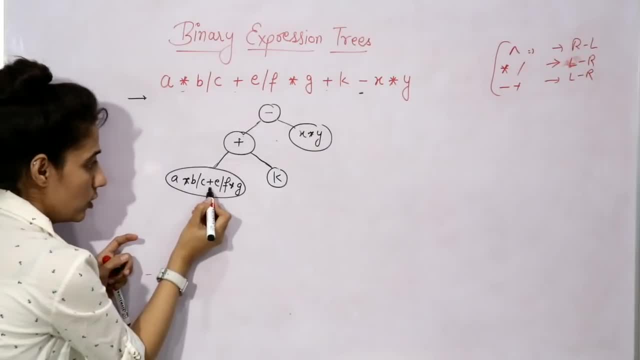 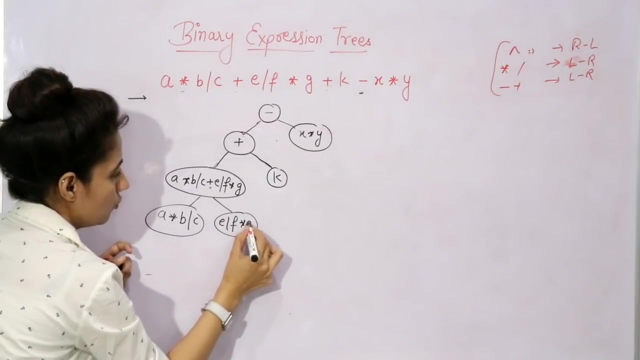 going to split this expression. So obviously this would be evaluated in the last Right. So this would be the root from here we are going to split this expression. So left part would be a asterisk b divide, c and right part of this plus would be e divide by f into g Right. So here the root would 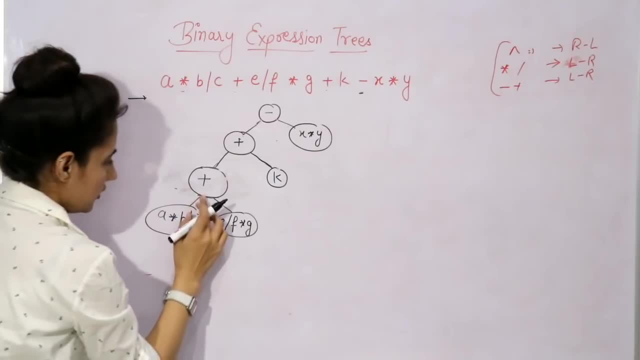 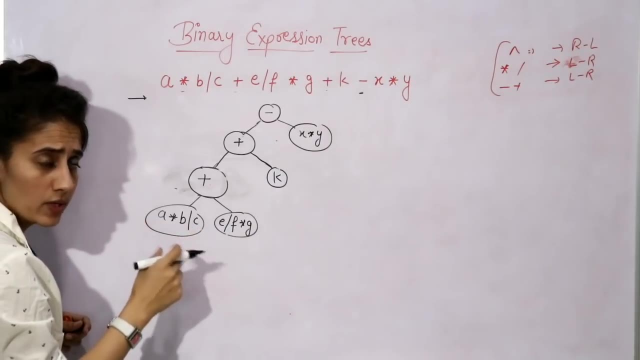 be only plus. Now. this is the tree. Now again, check for left and right subtree. We will make first of all the left subtree Here. also, we are going to split this expression. So left part of this is also following the same rule, because we are going to write down this coding in the loop Right. 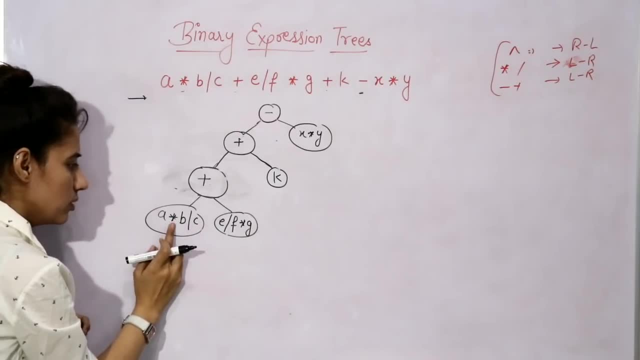 Now find out the operator which is having least precedence, But both multiplication and divide are having same precedence. Check out the associativity to resolve this conflict That is left to right. Now, from left to right, while scanning this asterisk, we find, and this would: 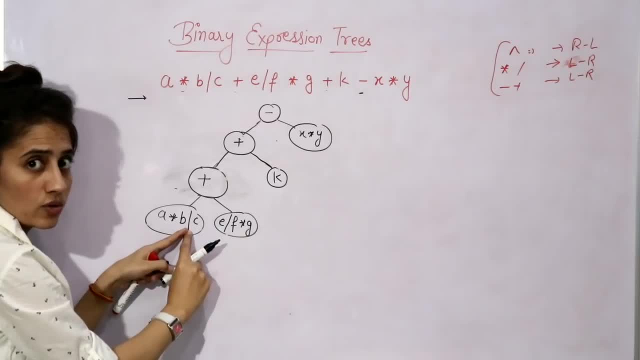 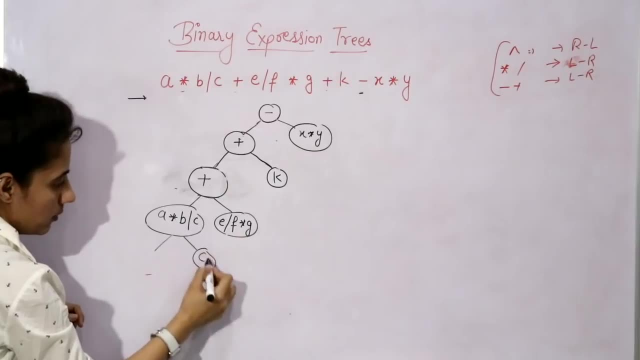 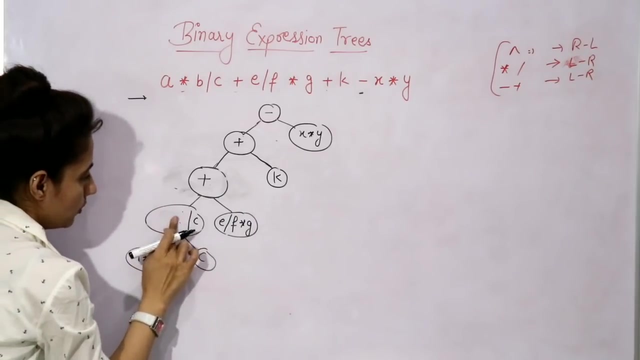 be evaluated first. After that we will evaluate this divide. So this is the last one which is going to be evaluated Now. split this expression. Right Part of this is would be c, and this is the left subtree. that is a asterisk b and the divide would be the root for. 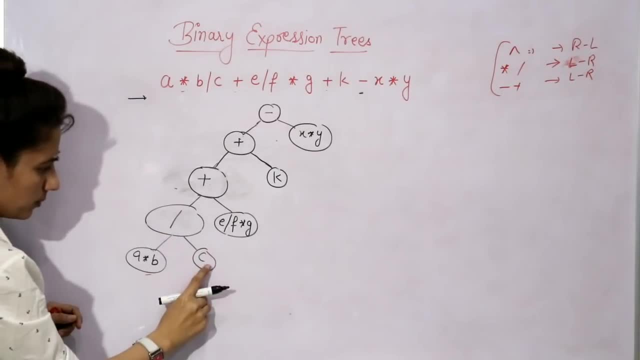 this subtree Right Now. here we have reached till the operand, So this is the leaf node. Now check out this one. Here we have only one operator, So no need to check out any precedence. Simply split it from here, asterisk, and the left would be a and right would be b. So we are done up to this Now. 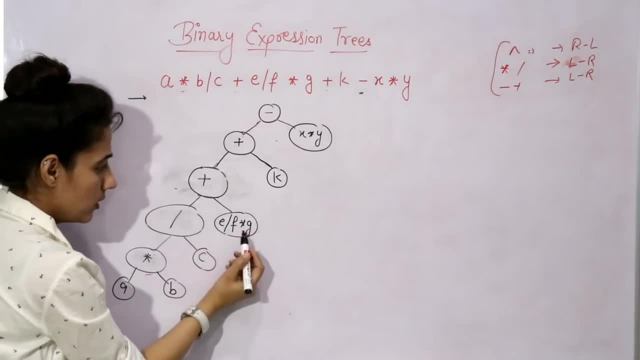 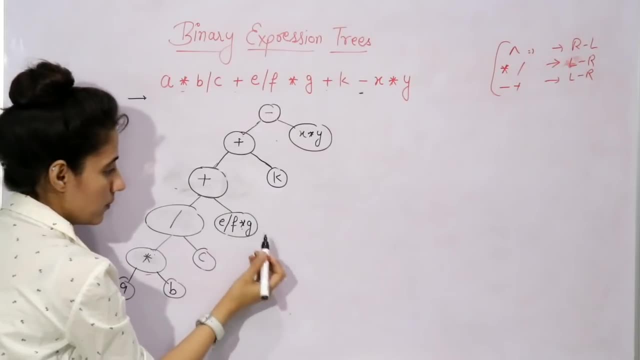 for this one. check out the precedence of the left subtree. So this is the left subtree, So this is the operator. Both are having same precedence. Associativity is left to right Now. this would be the last we are going to evaluate asterisk Right Now, here. we will split it from here, So this would 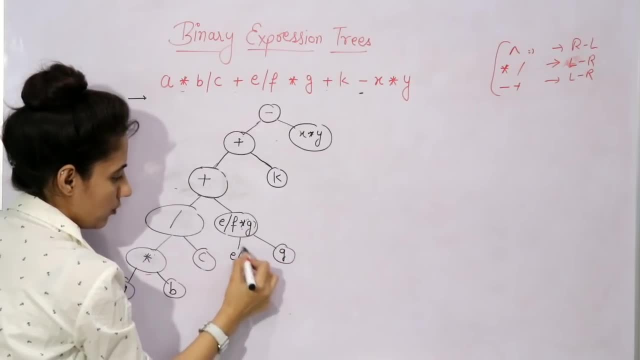 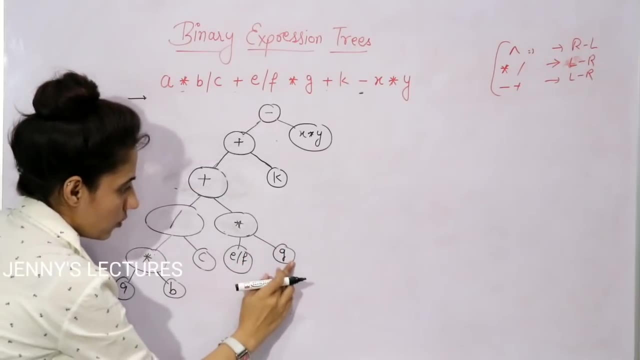 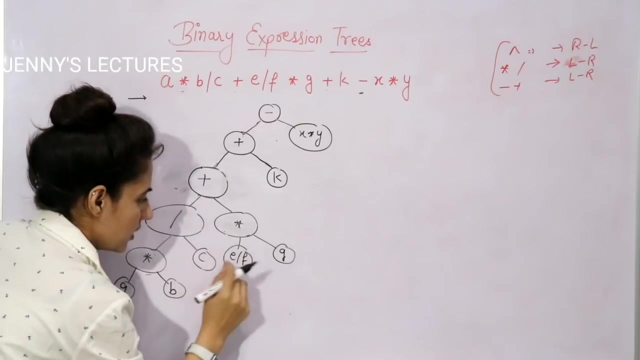 be the right subtree and e divide by f would be the left subtree for this one. So here the root for this is asterisk for this subtree. Now, this is the leaf node. We have reached till the operand E divide by f. Here we have only one operator. No need to check out any precedence, Simply. 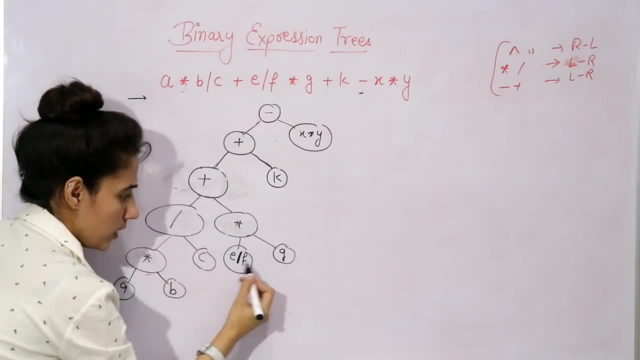 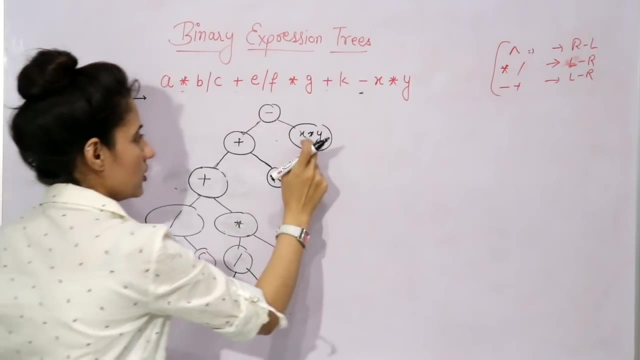 split the root. This: this would be from here. we are going to split this. So e would be to the left and f would be the right child for this one. So here we have divide. Now we are now check out this one. Here also we have only one operator, So no need to check out any precedence. So the 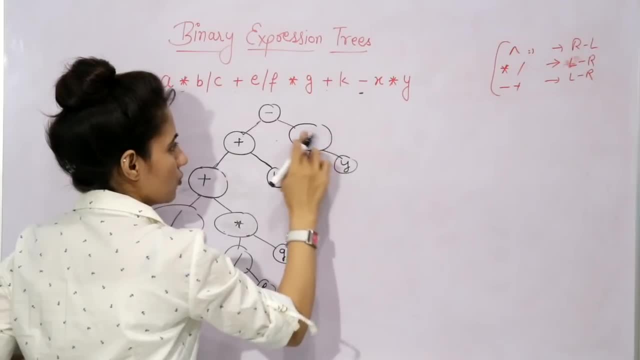 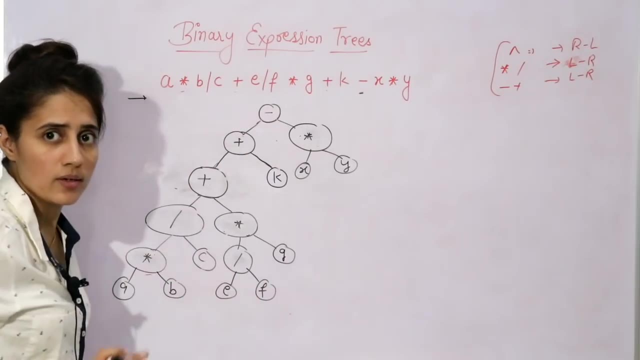 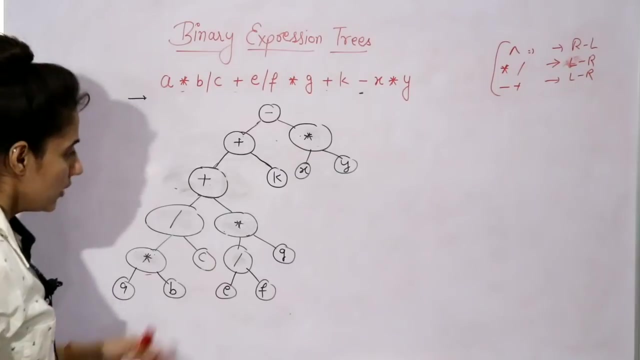 right child would be y, The left child would be x. So here we have asterisk Now for this in fix expression. this is the expression tree, So we haven't converted it into postfix and we have a constructed a expression tree. Now you can easily find out the prefix and postfix for this infix. 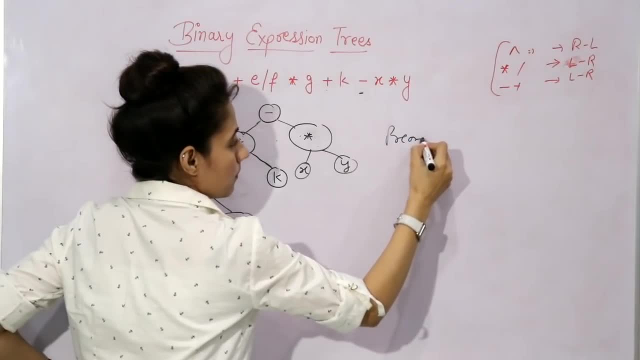 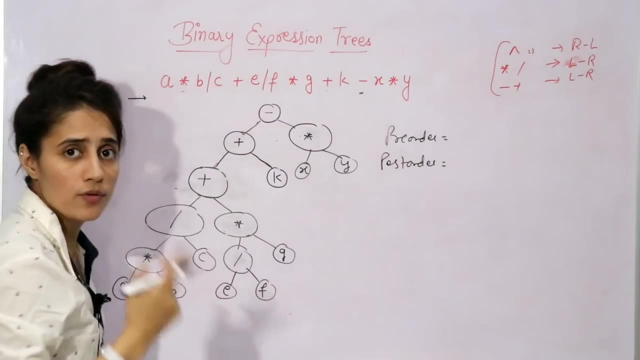 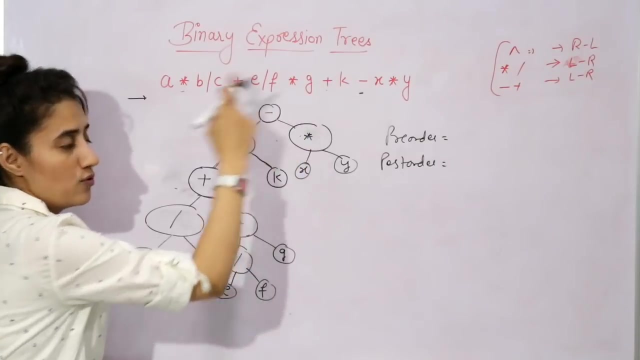 How, See, find out the preorder and postorder traversal Right For this tree. The preorder traversal of this tree would give you prefix expression for this infix and the postorder traversal of this tree would give you the postfix expression for this infix expression. Fine, So now I guess how to find. 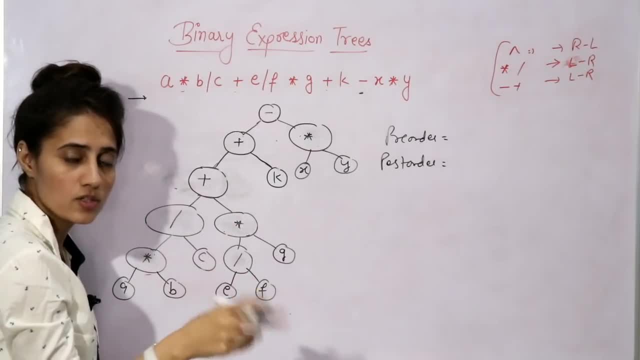 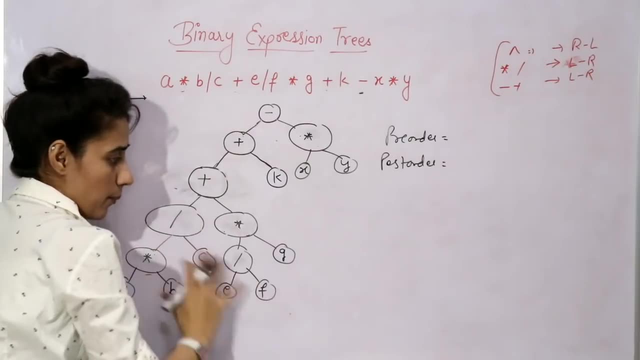 out the preorder, postorder and inorder. traversal of a tree- That thing we have already discussed. You can check out that video here. I am going to write down here the preorder and postorder. Fine, If you want to compare your answer, If you want to tell your answer, then you can construct, Then you 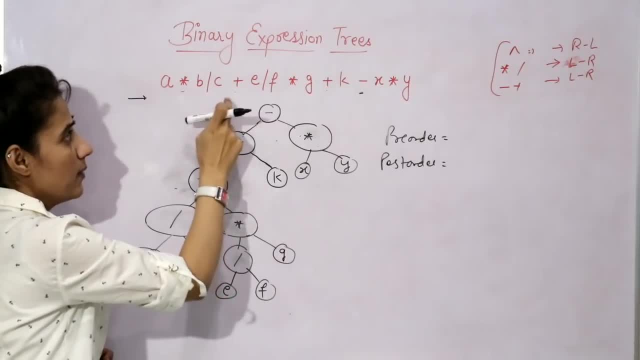 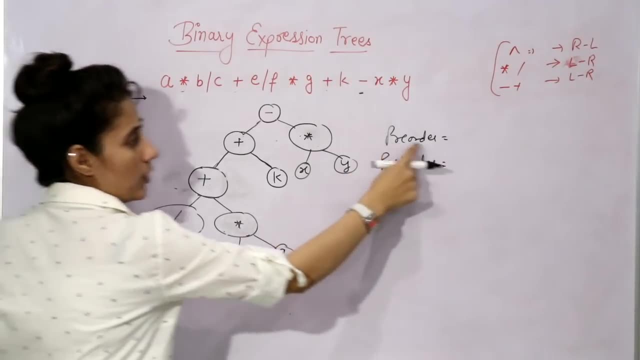 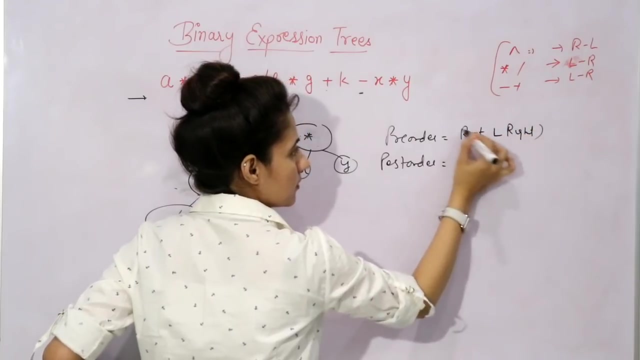 can find out the inorder traversal of this tree and if the inorder is same as the given infix, then you can say: this is the right tree, you have Right binded tree you have constructed Fine. So in order means left then right and right. Post order means here you will write left then right and 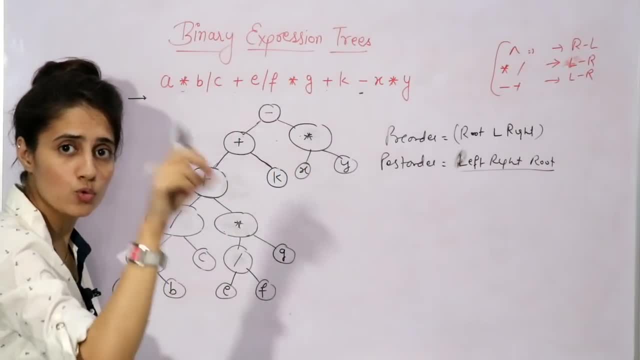 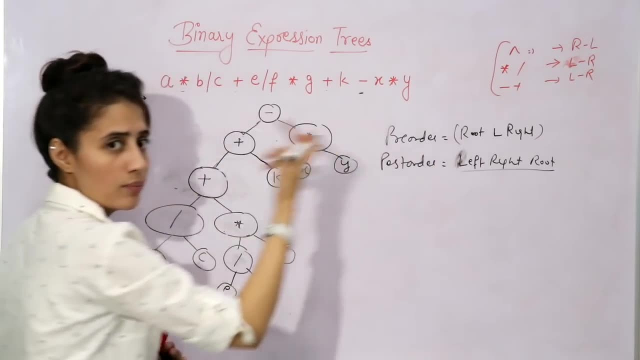 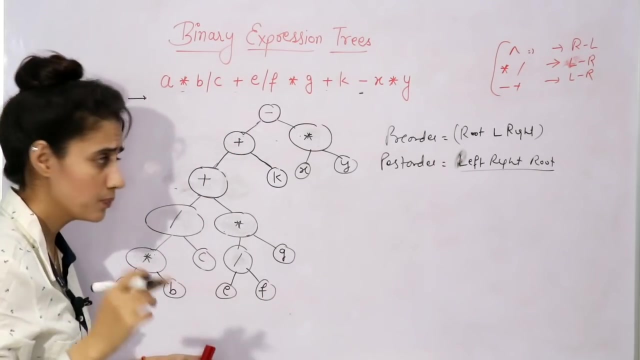 then route For inorder: left route right, Right, So ones to pre. Pre means first, it means route would be before left and right. Post order: post means later. It means route would be after left and right. Fine, In order. In means in between. Route would be in between left and right. 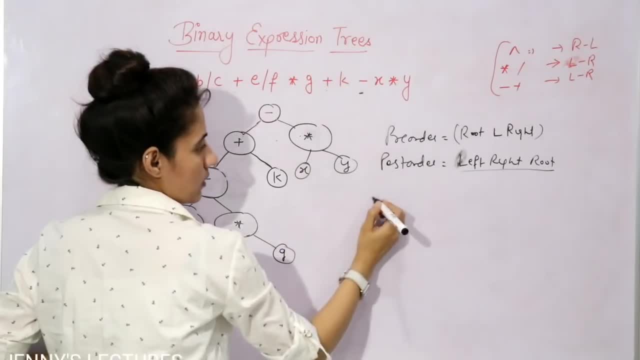 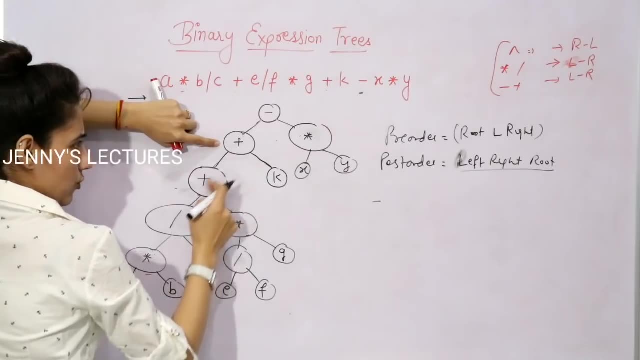 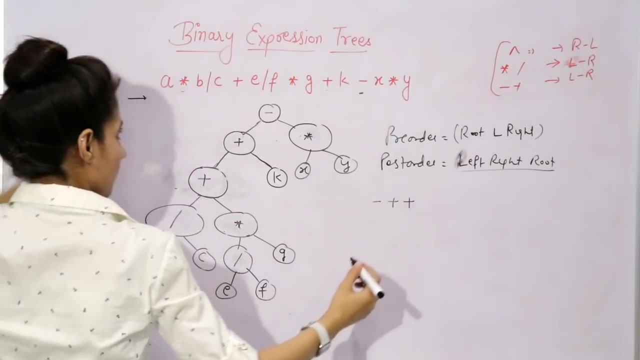 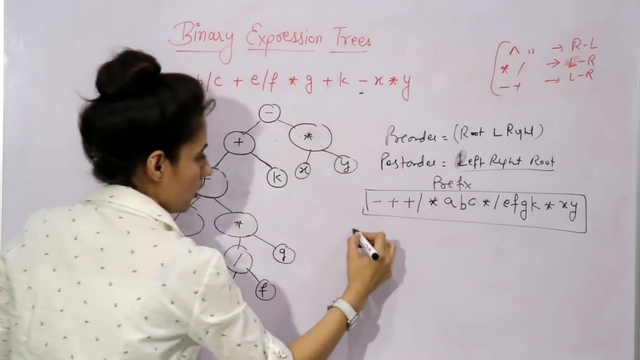 So now pre-order: find out the root. root is this minus. then left and right go to the left right, but this is again root for these child. so here you will write plus, then again here plus. so this is the prefix for the senfix expression. Now what about postfix? So this is the postfix.